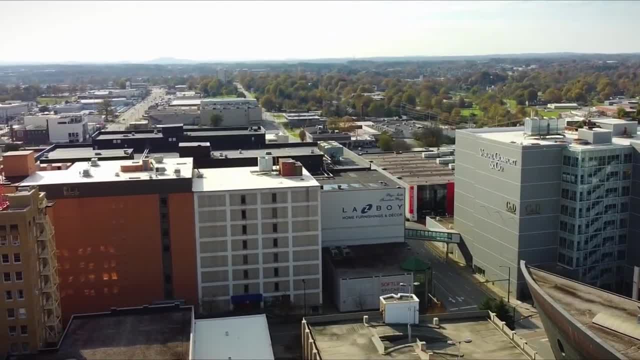 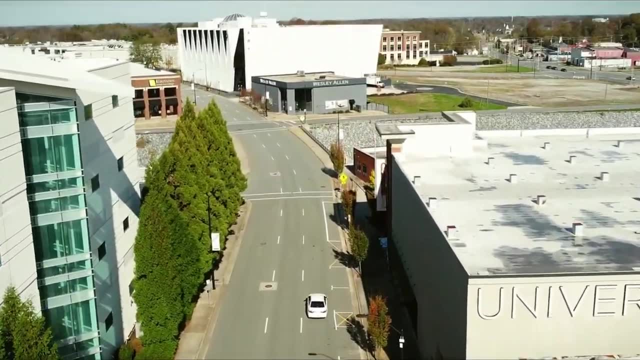 Triad region. It is consistently recognized as a terrific place to live, and it also has many attractions that draw in visitors from all over. This city is primarily known for being the home furnishings capital of the world. High Point and the surrounding area have over 100 furniture. 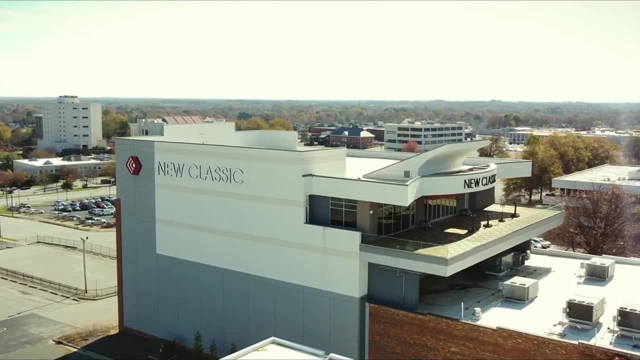 stores and outlets, as well as both the world's largest home furnishings show and the biggest furniture show. High Point is a city of the world's largest home furnishings show and the biggest furniture store, Whether you need to outfit an entire home or just find the perfect finishing. 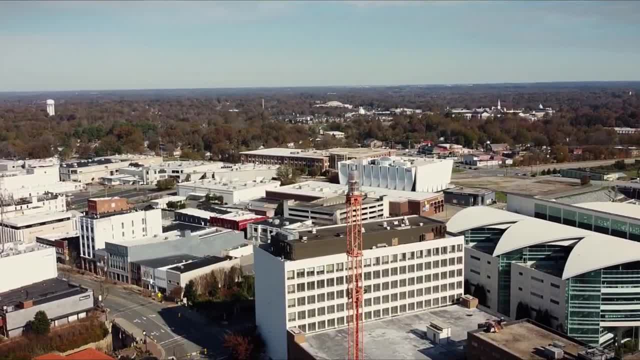 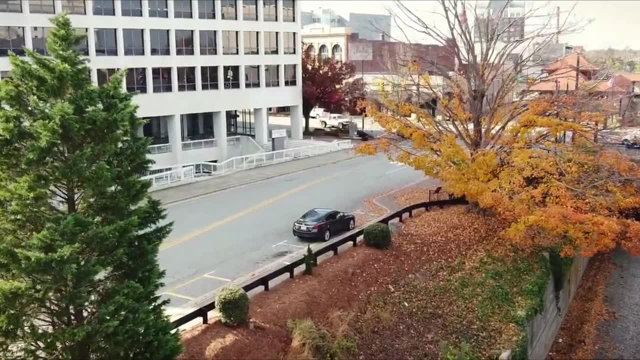 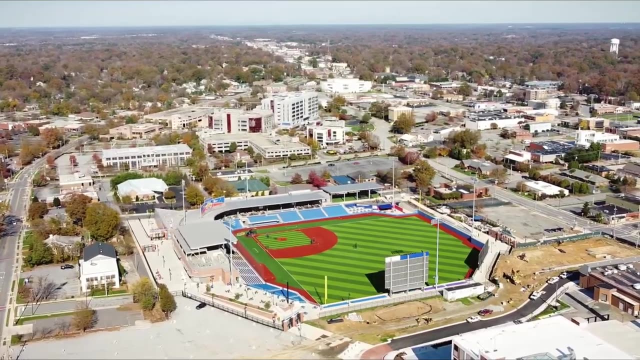 touches, High Point is the place to go. The city is not just about furniture. it also offers many fun experiences. Learn about the area's involvement with the Underground Railroad at the High Point Museum, Play laser tag and enjoy a high-ropes course at Kersey Valley Attractions. Watch a. 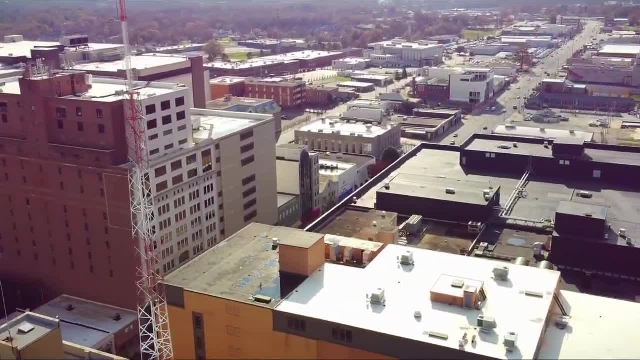 High Point Rockers game at Truist Point Stadium. You can even bring your dog to one of the city's pet-friendly breweries. High Point is a city of the world's largest home furnishings show. and the world's largest home furnishings show. You can even bring your dog to one of the city's pet-friendly breweries and parks. Number 8. Wilmington, North Carolina. Wilmington is the only coastal city that is also one of the state's 10 most inhabited cities. It has a population of around 115,451, according to the 2020 census, and many tourists come to experience some of the best nearby beaches. 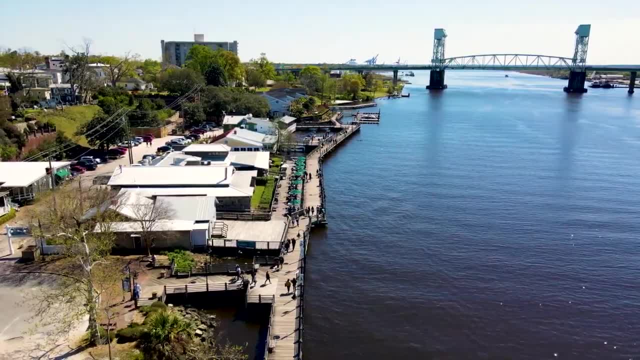 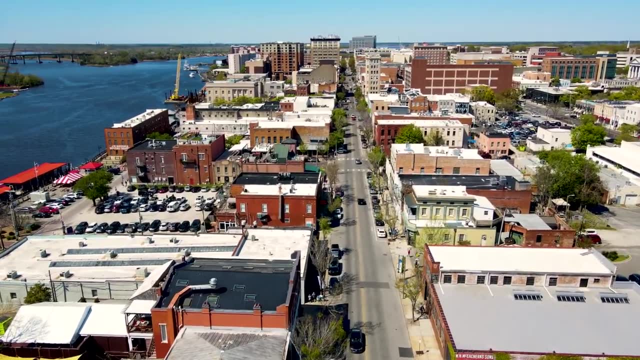 in the state There are three significant island beaches just a quick drive away from Wilmington. Wrightsville Beach is high-end and luxurious, as well as one of the world's best surfing destinations. Cooray Beach is calm and offers small-town, family-friendly vibes and a great beach area. 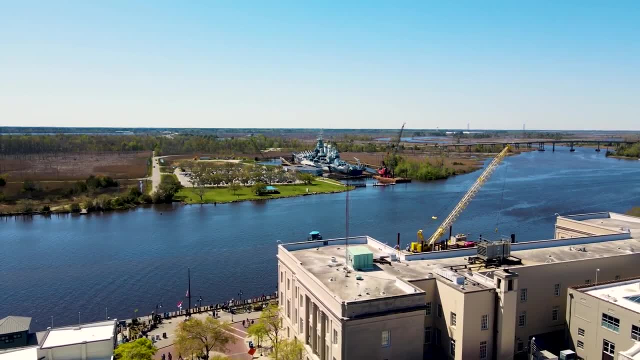 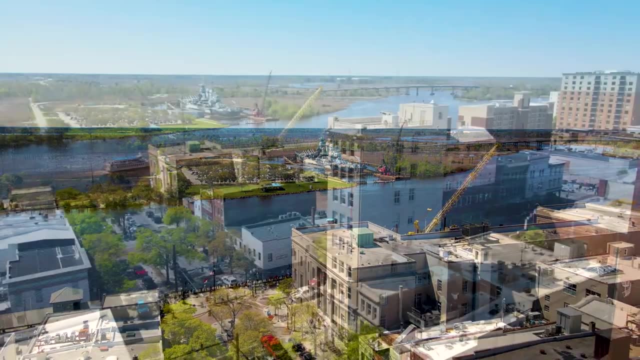 Carolina Beach is entertaining and an exciting beach town, complete with a beachside boardwalk, fun festivals and a state park. Despite being the hub for so many beach vacations, Wilmington itself has a calm, residential feel. Locals enjoy their long hot summers- easy beach access. 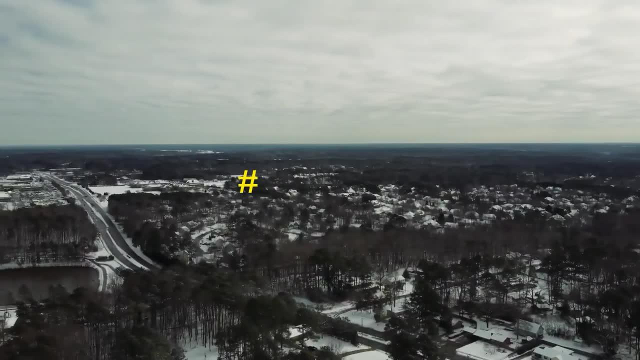 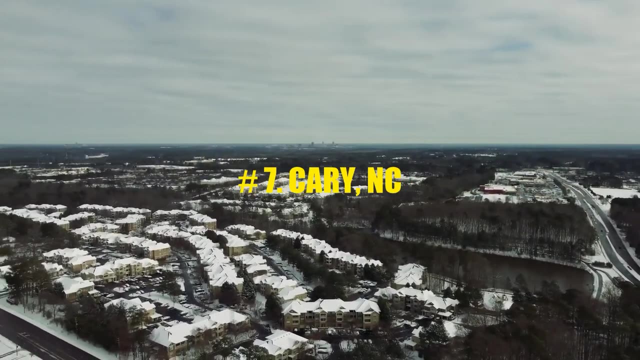 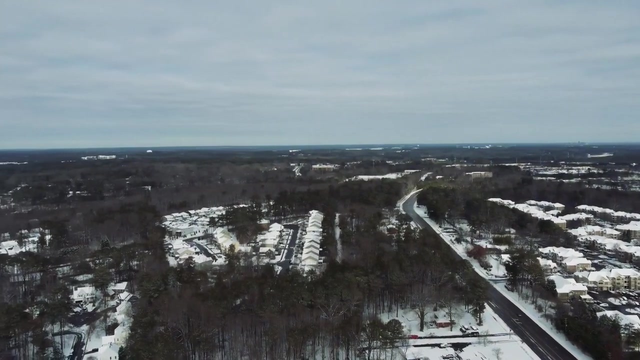 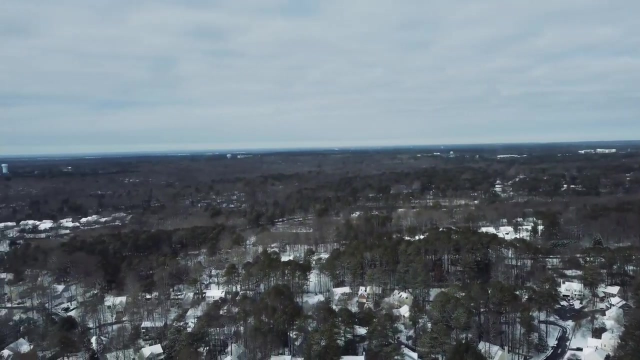 outdoor dining and friendly neighbors. Number 7. Cary, North Carolina. As a suburb of Raleigh, Cary provides proximity to everything in the state capital, as well as its own opportunities. Cary had a population of 174,721.. Because it is located in the Triangle area, staying in Cary is an ideal home base for 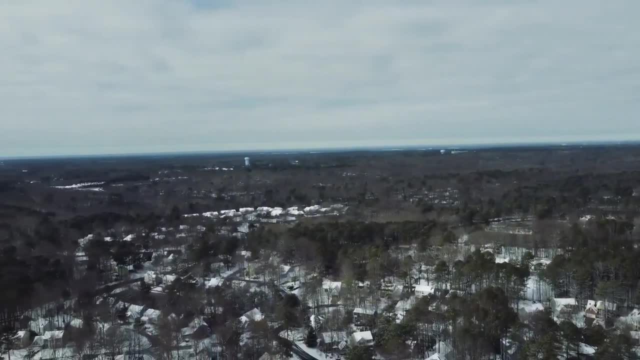 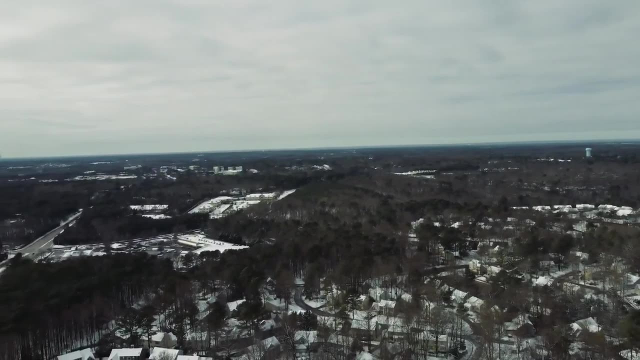 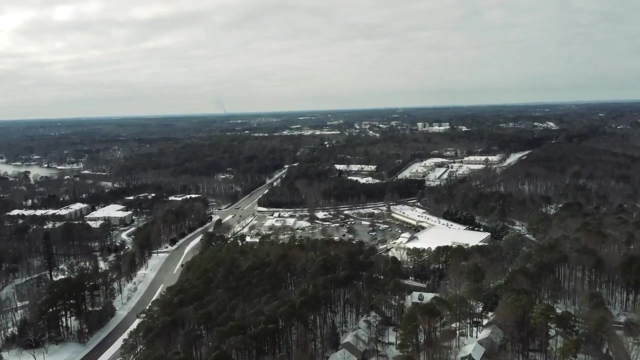 seeing everything in Raleigh, Durham and other nearby cities. It's a quick 15-minute drive into Raleigh and the two cities are also easily connected by the bus. Cary has several activities that make it a great place to live or visit. It has several sports facilities, including the USA Baseball National Training Complex. and the Wake Med Soccer Park, where various professional soccer teams play. The Coca Booth Amphitheater hosts events and performances within nature. Cary is also home to the North Carolina Symphony during the summer months. Number 6. Fayetteville, North Carolina. Fayetteville is a city in the state of North Carolina. It is a city of the North Carolina. 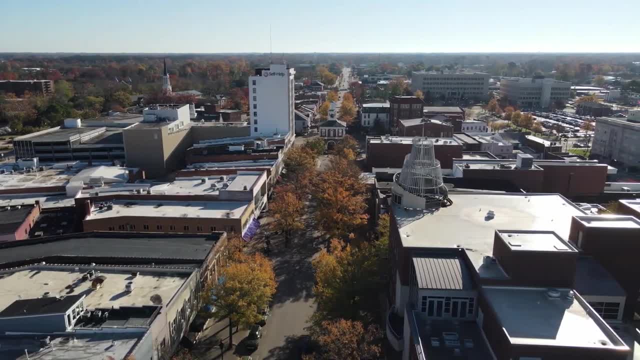 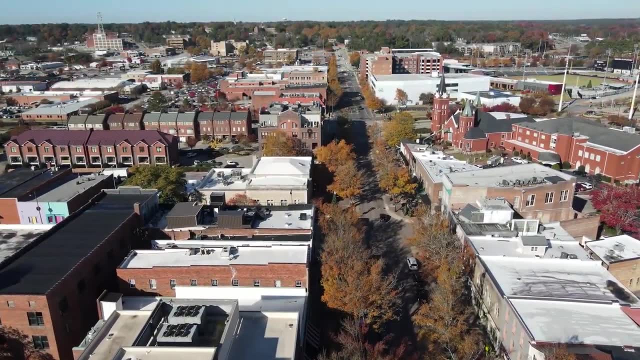 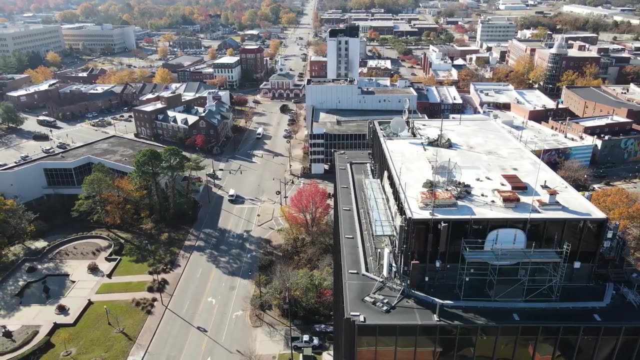 City about 60 miles south of Raleigh, with roughly 208,501 residents according to the 2020 census. It has many shops, museums, events and more, as well as a strong suburban and homing feel for its community. The city's community puts on various events throughout the year in Fayetteville. 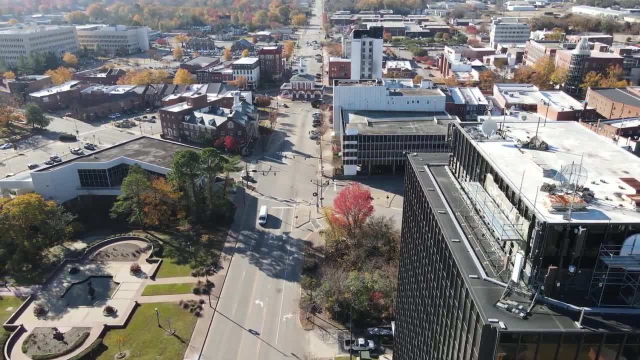 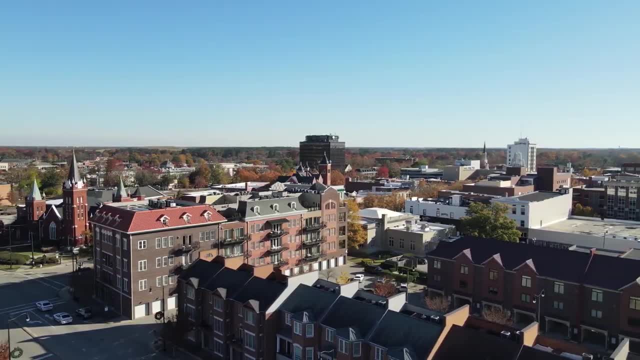 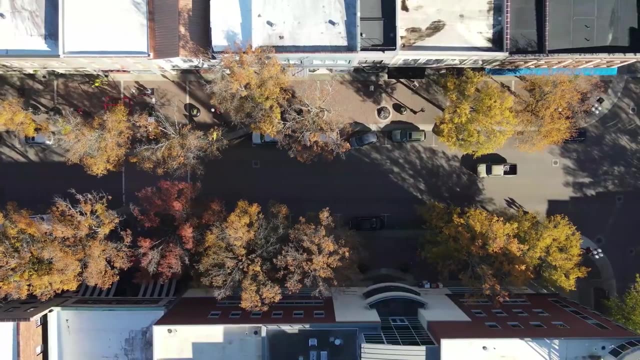 The International Folk Festival is an annual multicultural event that celebrates diverse arts and cultures. The Fayetteville Dogwood Festival organization puts on a variety of family-friendly festivities, including Fayetteville After Five, the Miss Fayetteville Pageant and the Spring and Fall Fayetteville Dogwood Festivals. Tourists often enjoy checking out. 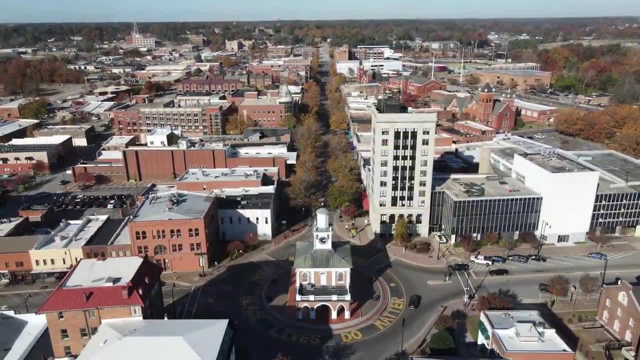 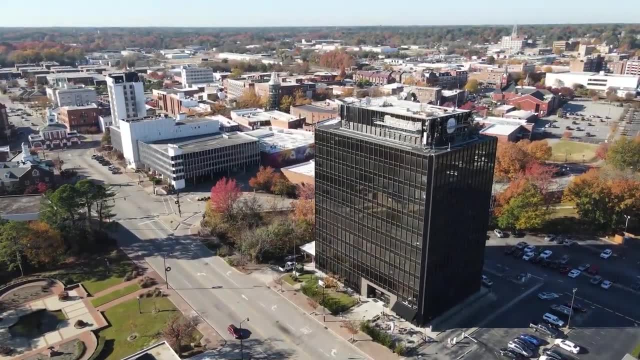 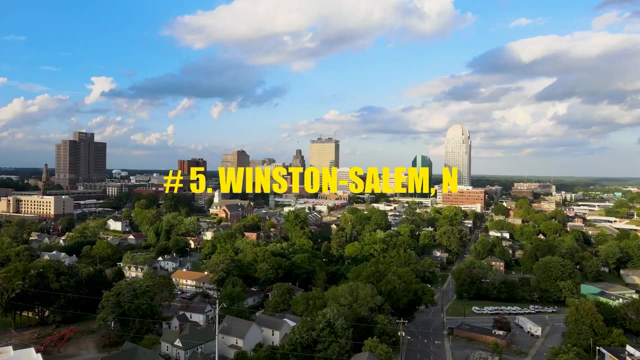 Fayetteville's museums as well. The Airborne and Special Operations Museum teaches about the US Army's history, and the Museum of the Cape Fear Historical Complex focuses on cultural heritage in the local area Number 5.. Winston-Salem, North Carolina, Located about a 30-minute drive west of 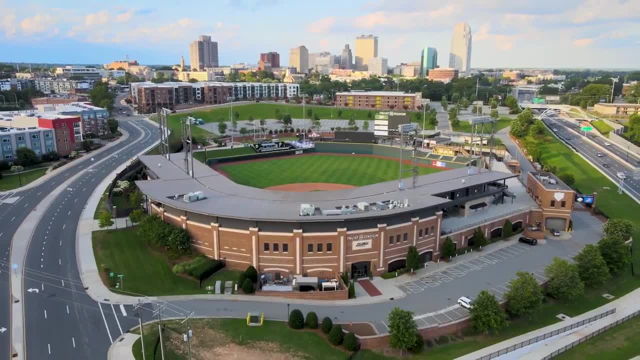 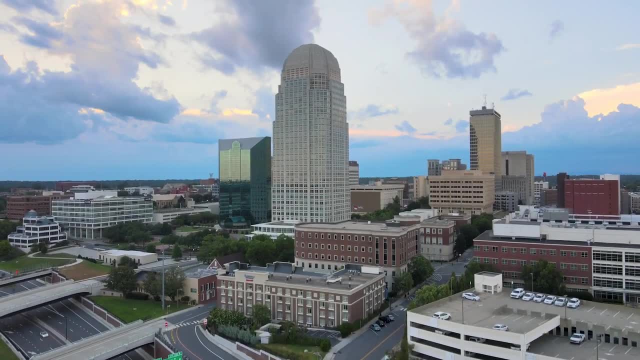 Greensboro. Winston-Salem has just under 250,000 residents. Its location in the Piedmont Triad region makes it a great home base for experiencing beautiful nature in the surrounding area, as well as the city's own unique history and attractions. Winston-Salem is often known as: the Twin City. In 1913, Winston and Salem, two towns just a mile apart, officially merged to create what we now know as Winston-Salem. This united city also has a notable history of being involved in the tobacco industry, particularly Camel Cigarettes, giving Winston-Salem its second. nickname the Camel City. Old Salem is now a charming historic downtown area. It has many shops, gardens, cafes and other attractions to explore. The entire area also serves as a museum that teaches about the history and culture of Moravians in the area Number 4. Durham North. 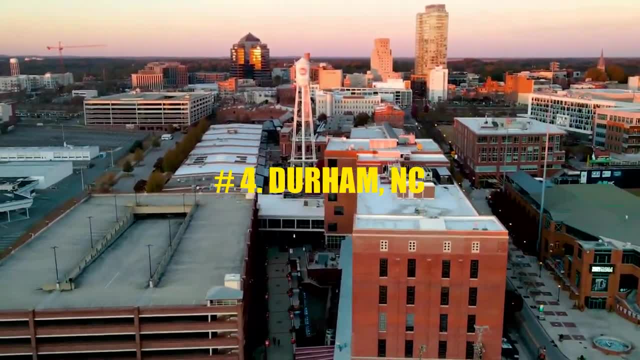 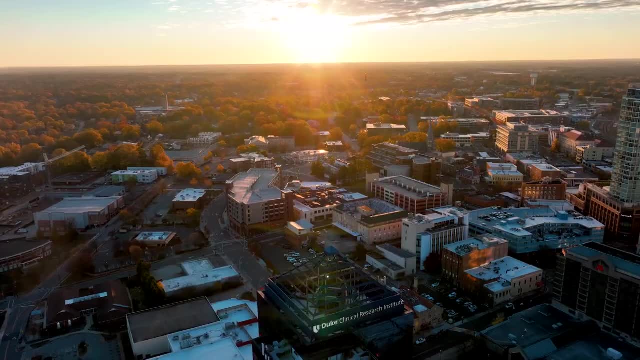 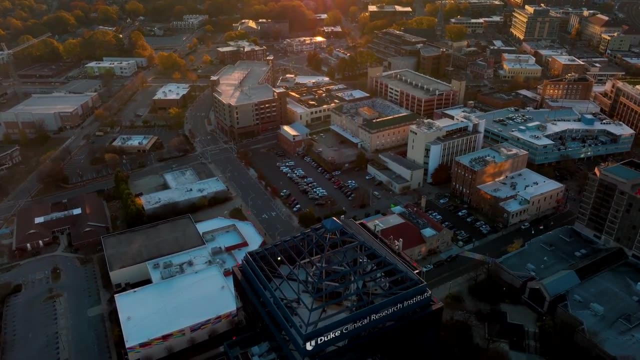 Carolina, Durham. the Bull City is a quick 30-minute drive west of Winston-Salem and is a from Raleigh and another integral part of the Research Triangle. It had a population of 283,506 people. Durham's major academic institution is Duke University, a private research university. 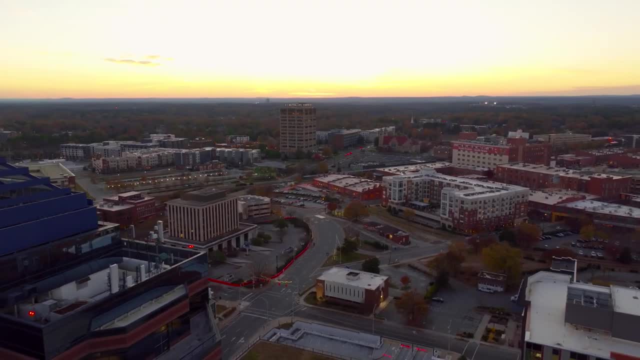 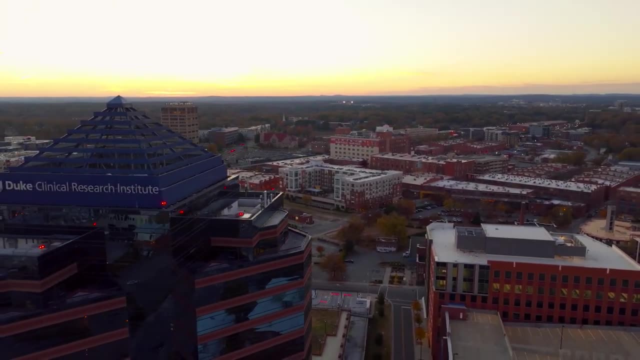 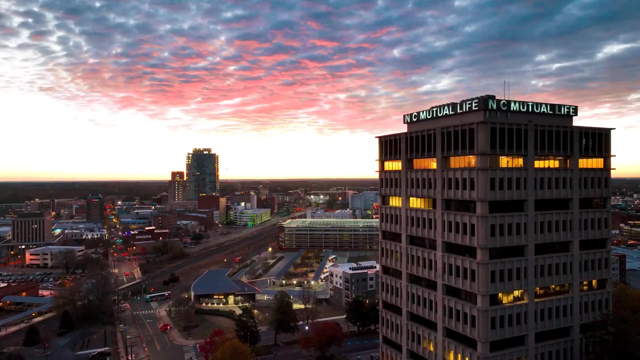 ranked the 10th-best national university by the US News & World Report in 2022. It attracts stellar students from across the world to come to Durham for their studies. Other colleges and universities in Durham include North Carolina Central University and Durham Technical Community College. Shopping opportunities. 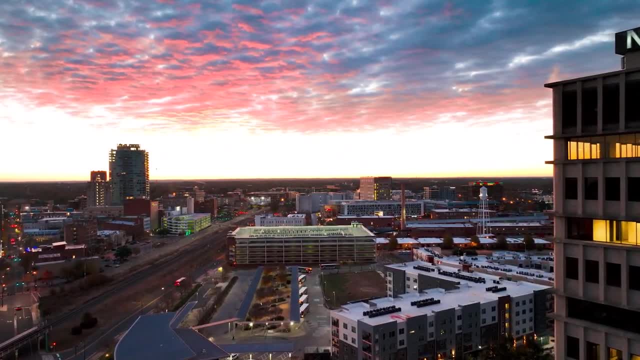 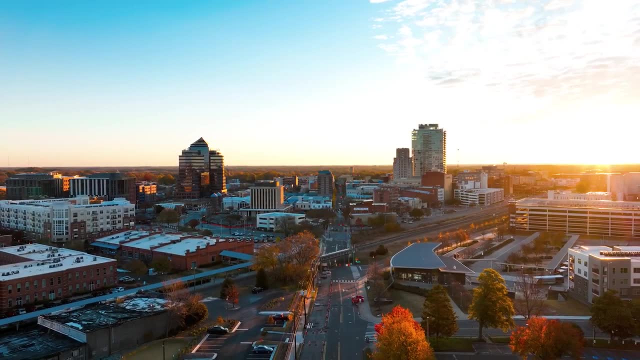 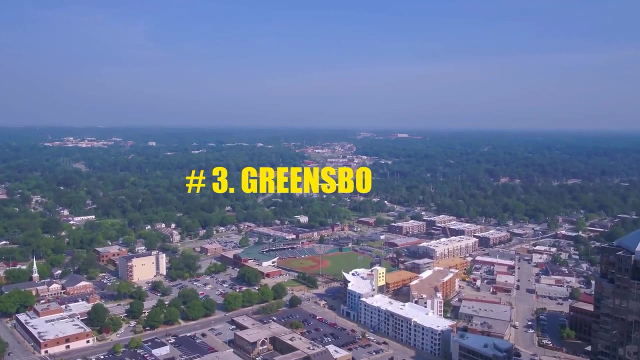 also attract people to the city. The Streets at South Point is a large shopping center with over 150 shops and many restaurants. Downtown Durham has numerous boutiques and shops for people who want more local options. Number 3. Greensboro, North Carolina. 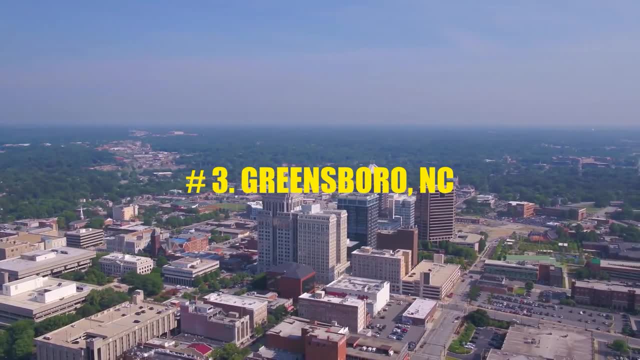 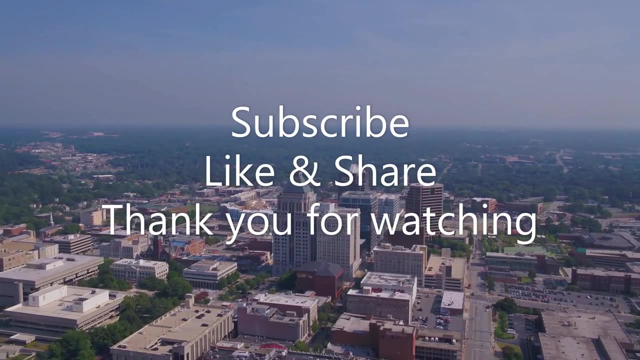 Located in northern North Carolina, Greensboro has around 299,035 restaurants, restaurants and restaurants. Its central location makes it an easily accessible destination for North Carolinians, especially those in the Raleigh-Durham area, as well as many Virginians. 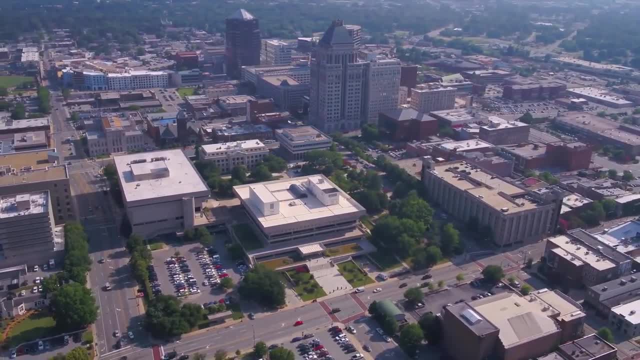 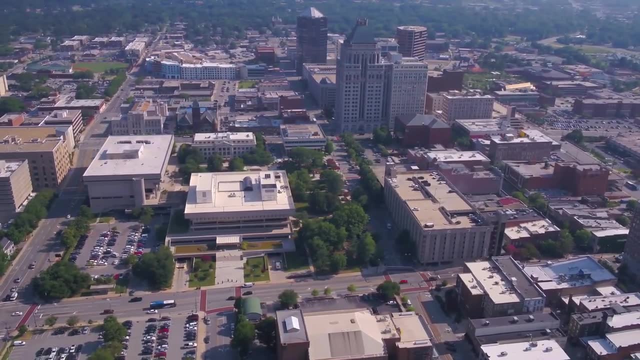 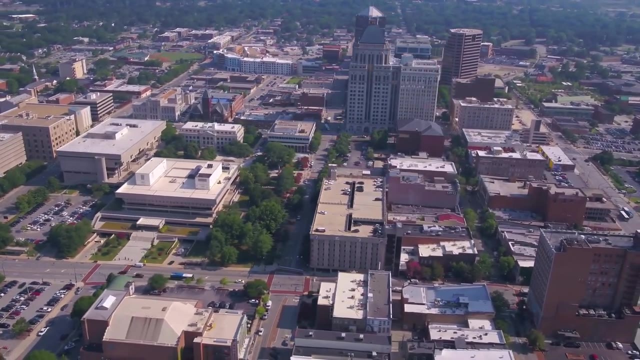 Downtown Greensboro is undoubtedly one of the city's most important areas. Its historic buildings and overall charm create an ambience perfect for window shopping at boutiques and finding a bite to eat at a cafe or restaurant. Additionally, the downtown area has tourist attractions such as the International Civil Rights Center and Museum and the City of Durham. 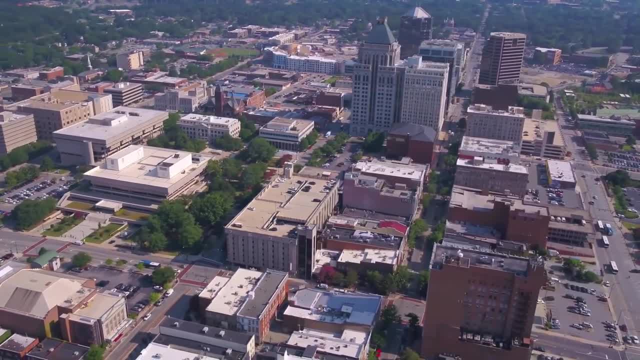 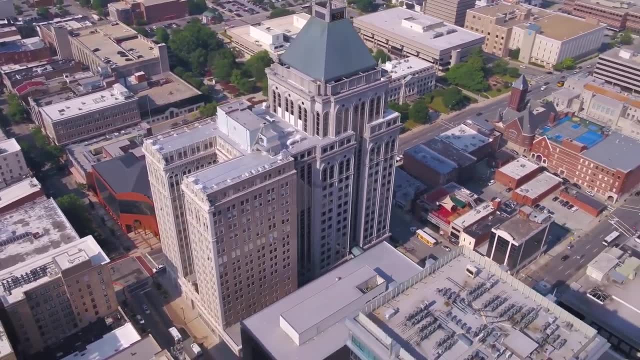 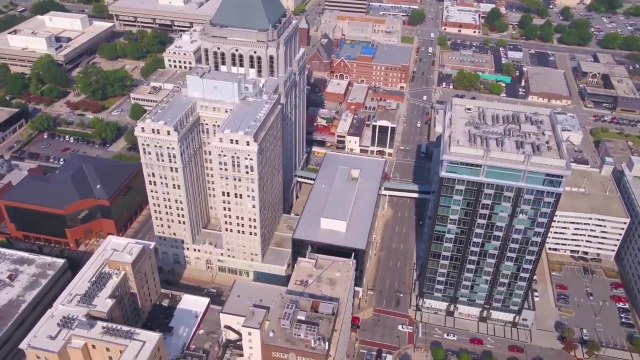 A can't-miss local attraction is the Greensboro Science Center. This impressive center includes a 12-acre zoo, an aquarium and a hands-on museum. It's an ideal place for the whole family to learn about science through interactive experiences. Number 2. Raleigh, North Carolina. 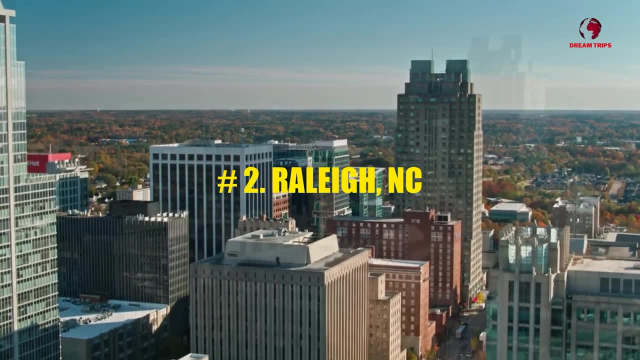 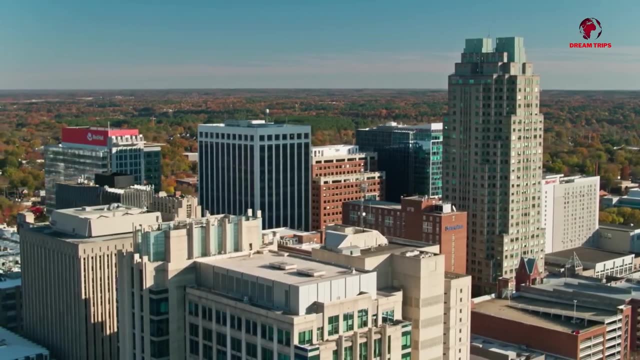 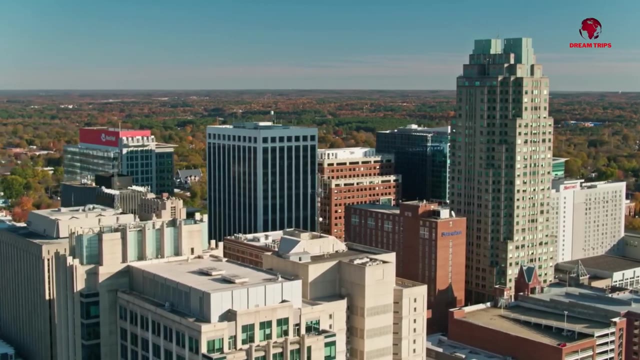 North Carolina's capital city is Raleigh, home to 467,665 residents and a common tourist destination. It's one of the state's most populated areas and an integral part of the Research Triangle, which recognizes the importance of Raleigh, Durham and Chapel Hill in the research. 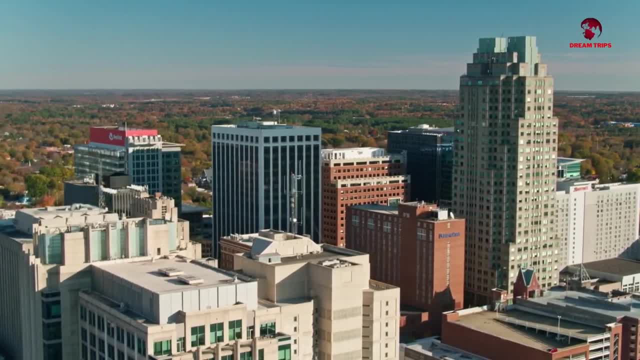 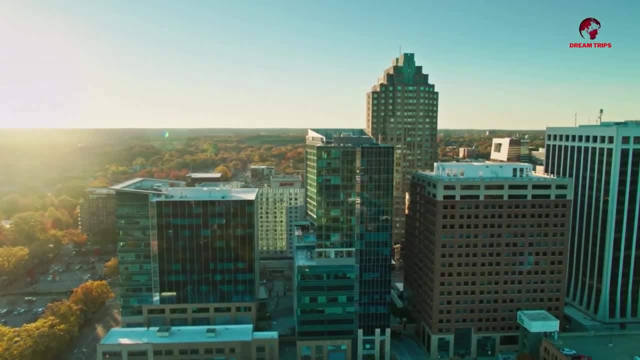 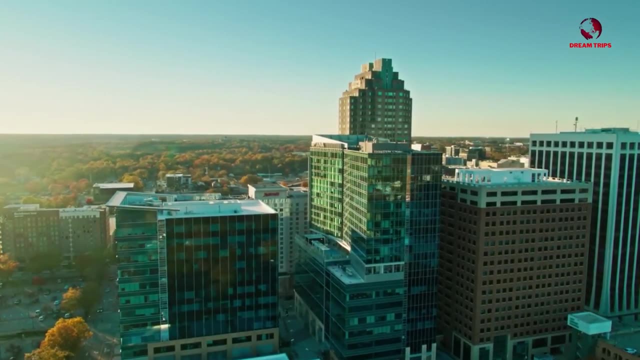 field. Raleigh, in particular, is well known for its academic institutions. North Carolina State University is NC's largest university, with over 36,000 students in 2022, and is especially highly regarded for its STEM education. Other colleges and universities in Raleigh include Meredith. 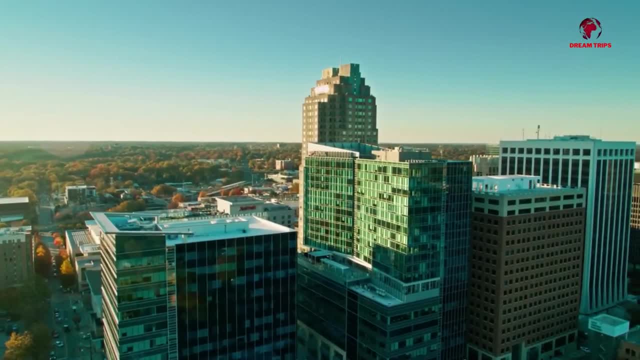 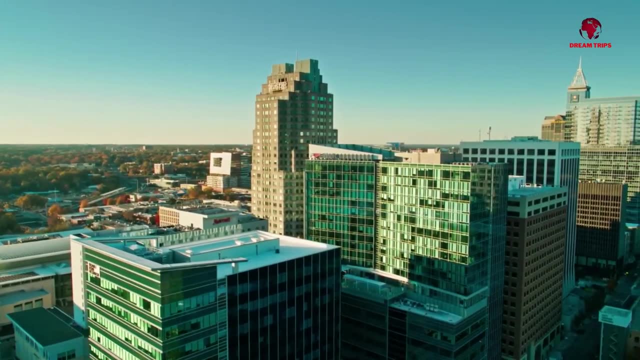 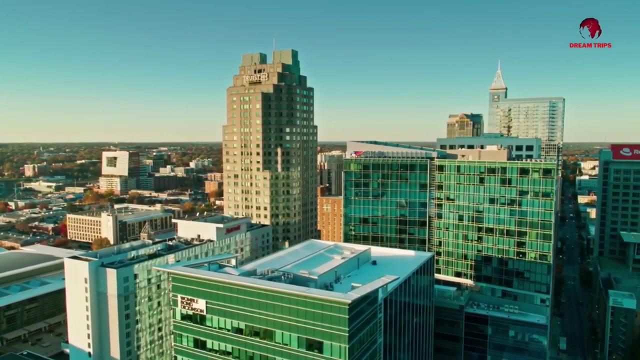 College, Shaw University and William Peace University. One of the state's most important historic sites, the North Carolina State Capitol, also resides here. It was completed in 1840 in a Greek Revival style of architecture and is a US National Historic Landmark Still the active. 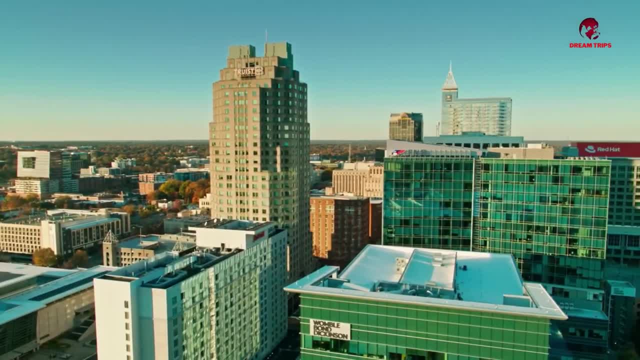 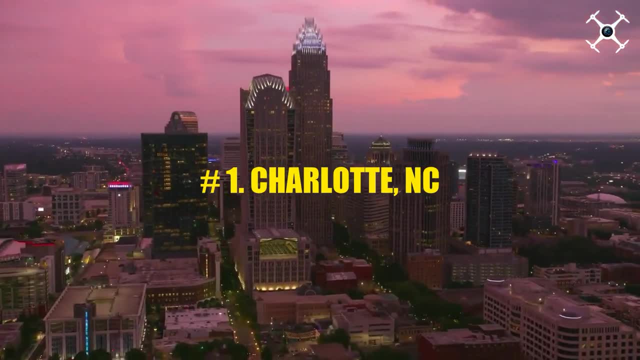 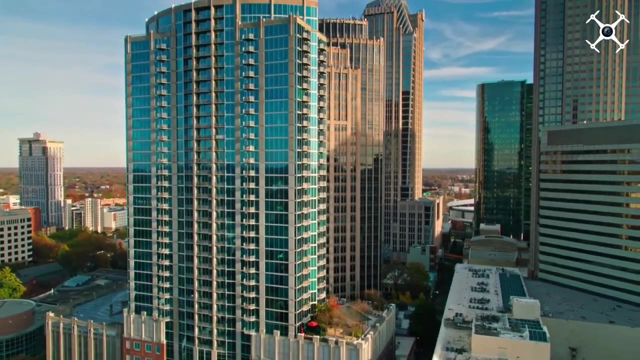 Capitol building. it's open for self-guided and guided tours. Number 1. Charlotte, North Carolina. The bustling business and entertainment hub of North Carolina, Charlotte is the state's most populous city. The Queen City had around 874,579 residents.